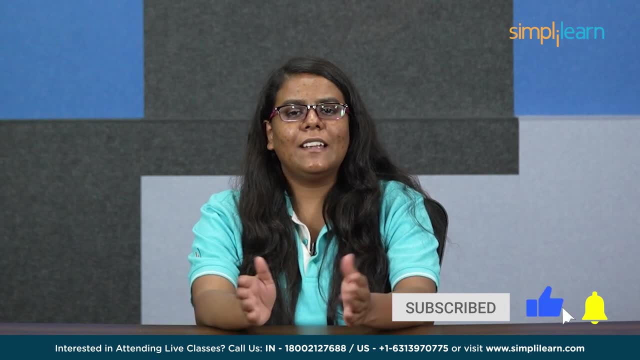 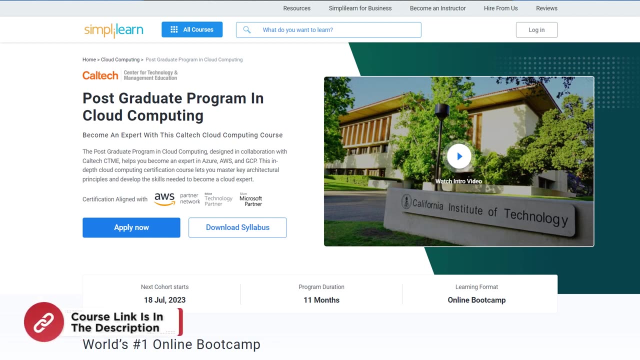 But before that, do subscribe to our YouTube channel and hit the bell icon to see more such interesting content in future. And if you want to learn more about these types of concepts and cloud computing services, then our Caltech Postgraduate Program in Cloud Computing will. 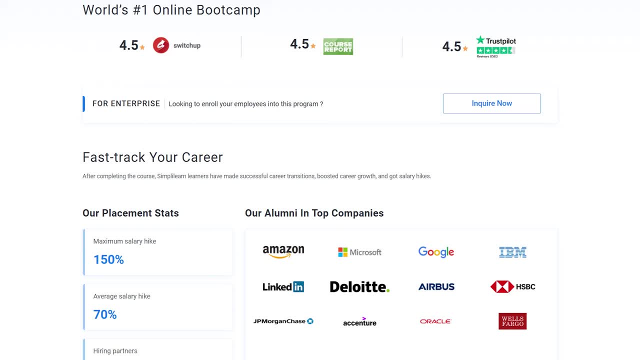 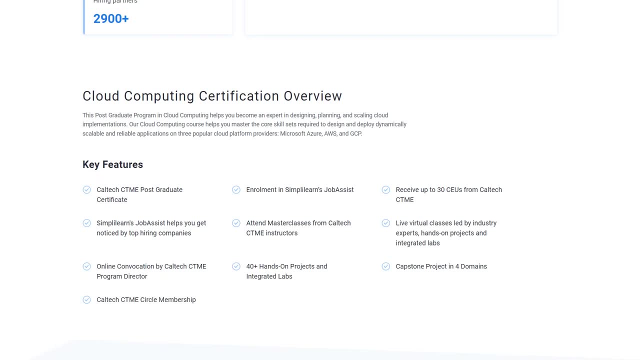 be the right choice for you. This postgraduate program in cloud computing will help you become an expert in Azure and AWS. This in-depth course lets you master key architectural principles and develop the skills needed to become a cloud expert. So if you are interested in, 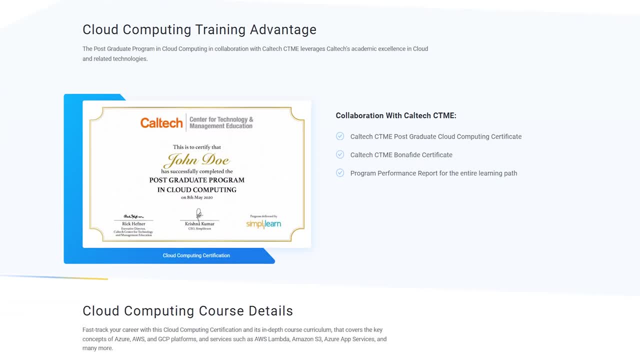 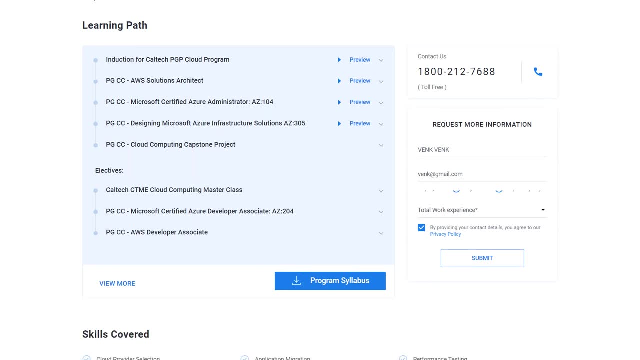 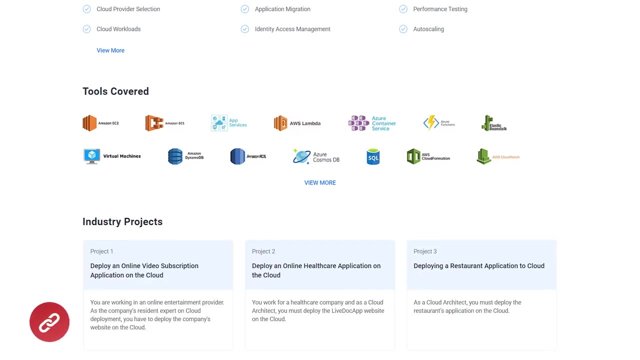 learning more about cloud computing, then you can click on the link in the description. It will help you become an expert in designing, planning and scaling cloud implementations. Our cloud computing course helps you master the core skillsets required to design and deploy dynamically scalable and reliable applications on Microsoft Azure and AWS. So do check out the. 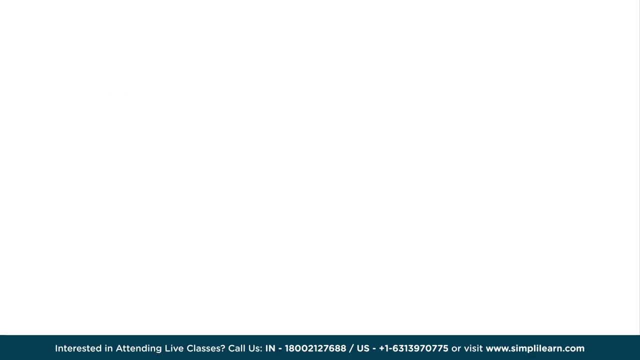 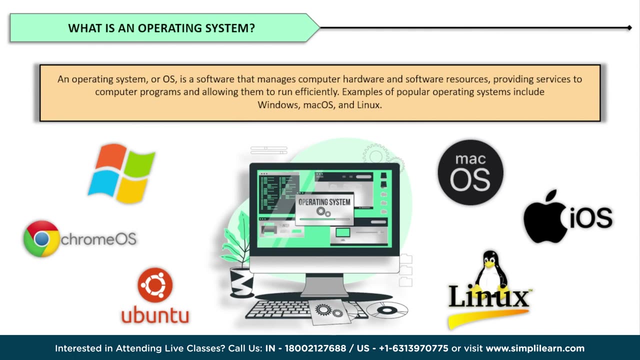 course link mentioned in the description. So let's get started. But before we delve into a real-time operating system, let's first understand what an operating system is. An operating system, or OS, is a software that manages computer hardware and software resources providing services. 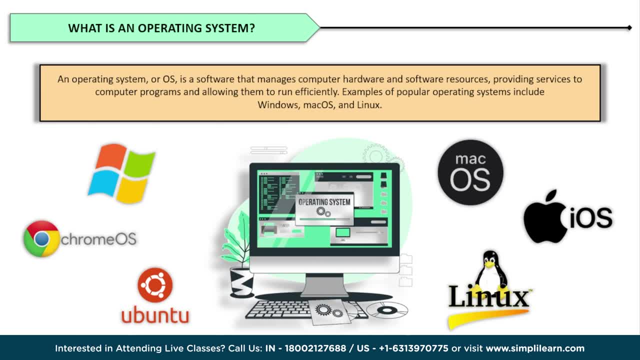 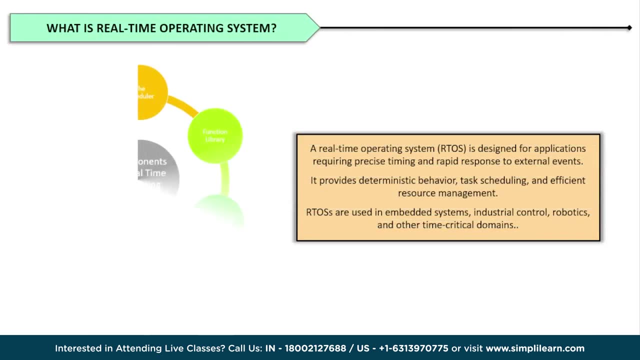 to computer programs and allowing them to run efficiently. Examples of popular operating systems include Windows, MacOS and Linux. Now, what sets real-time operating systems apart from regular operating systems? Well, the key distinction lies in the ability to respond to events in a deterministic and timely manner In a real-time system, meeting deadlines. 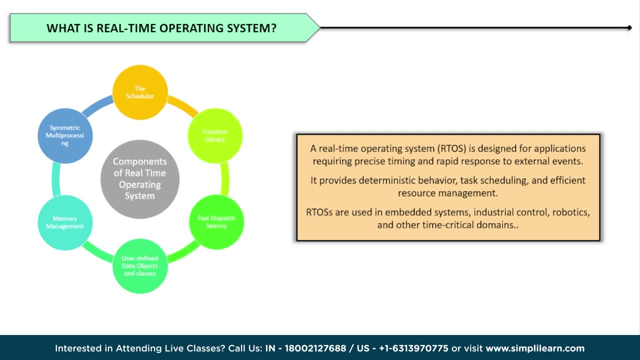 is of utmost importance. It must be able to complete tasks within specific time constraints, known as deadlines. Real-time operating systems find applications in various critical domains, such as aerospace, automotive, medical devices and industrial automation. These systems are designed to handle time-critical tasks and provide a predictable response. Imagine an airbag. 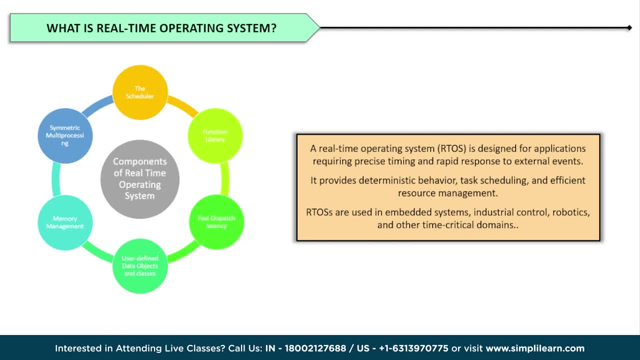 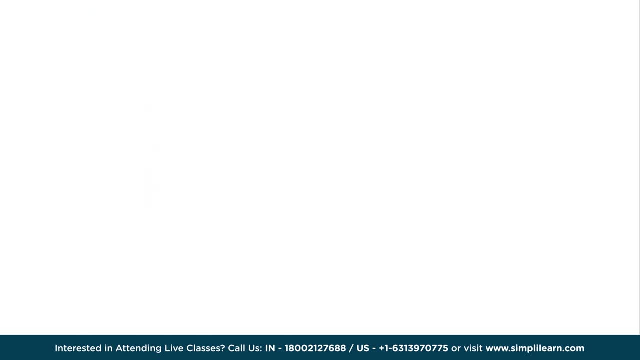 deployment system in a car. It needs to react instantly in the event of a collision. That's where real-time operating systems shine. Now let's discuss two types of real-time operating systems: hard real-time and soft real-time. In a hard real-time, missing a deadline can 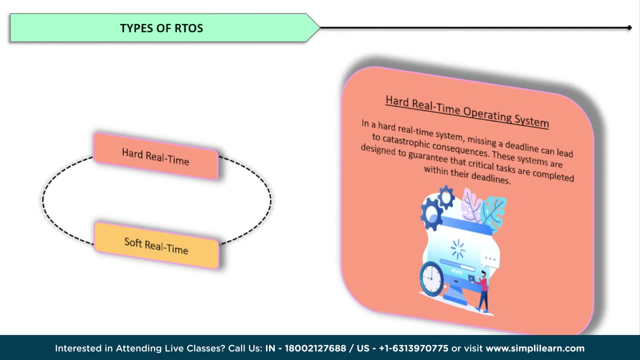 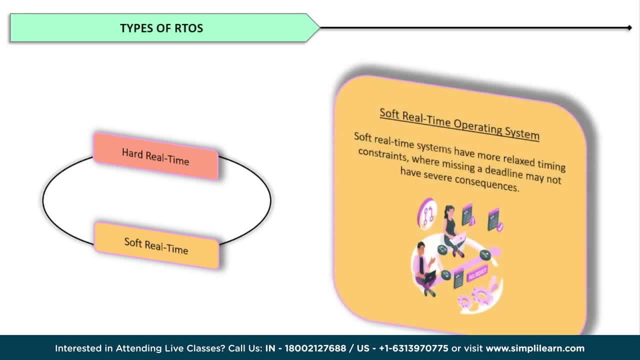 lead to catastrophic consequences. These systems are designed to guarantee that critical tasks are completed within their deadlines. On the other hand, soft real-time systems have more relaxed timing constraints, where missing a deadline may not have severe consequences. But real-time operating systems achieve this goal. Real-time operating systems are designed 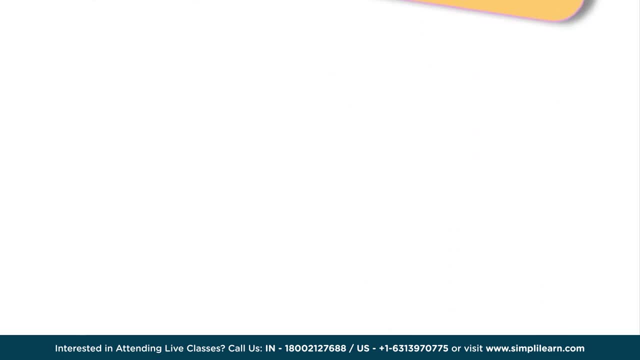 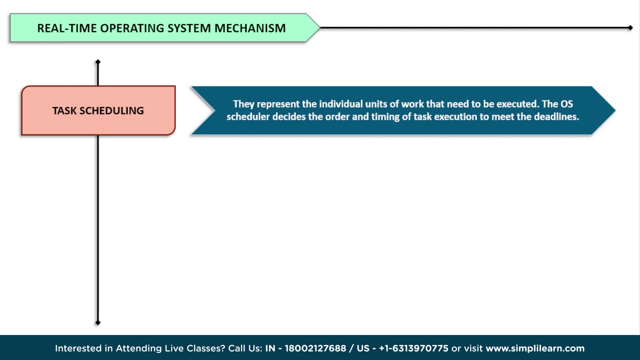 to handle time-critical tasks and provide a predictable response. Real-time operating systems achieve their deterministic behavior through various mechanisms. One key component is task scheduling. Tasks are the building blocks of real-time systems. They represent the individual units of work that need to be executed. The OS scheduler decides the order and timing. 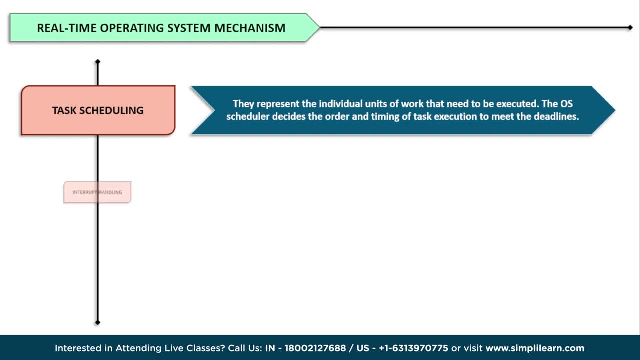 of task execution to meet the deadlines. Another critical aspect is interrupt handling. Interrupts are events that occur externally or internally and require immediate attention from the operating system. Real-time OS should respond to these interrupts promptly and prioritize them based on their urgency. Real-time operating systems also employ techniques like priority inversion. 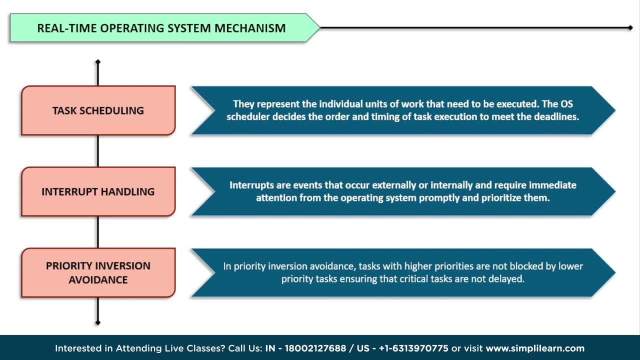 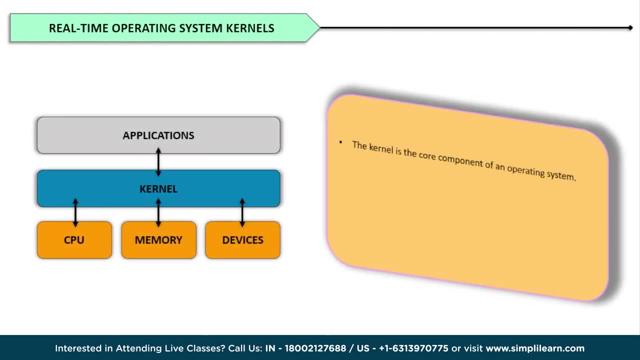 avoidance, where tasks with higher priority are not blocked by lower priority tasks. This ensures that critical tasks are not delayed or blocked by less important tasks. Now let's talk about real-time operating system kernels. The kernel is the core component of an operating system that provides essential information for the task. The kernel is the 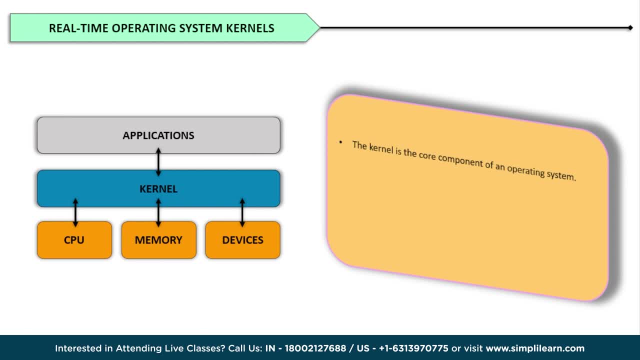 core component of an operating system that provides essential information to the task, essential services to applications and manages hardware resources. Real-time kernels are designed to handle time-critical tasks efficiently. They provide features such as fast context switching, minimal interrupt latency and deterministic task scheduling. One popular real-time operating system is 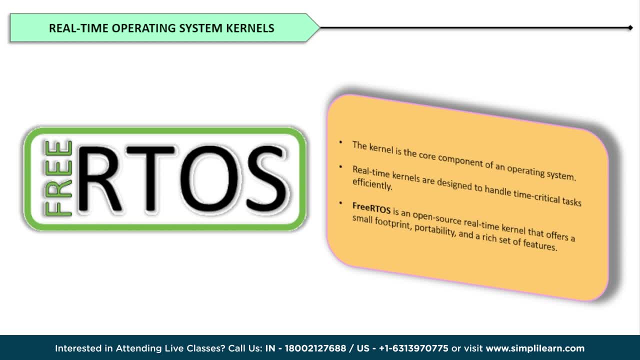 FreeRTOS. It's an open-source real-time kernel widely used in embedded systems. FreeRTOS offers a small footprint, portability and a rich set of features. It's a great choice for resource-constrained devices where efficient task management is crucial. Now let's explore some real-world examples of 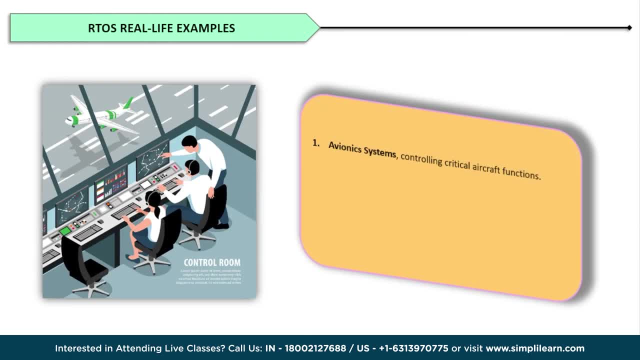 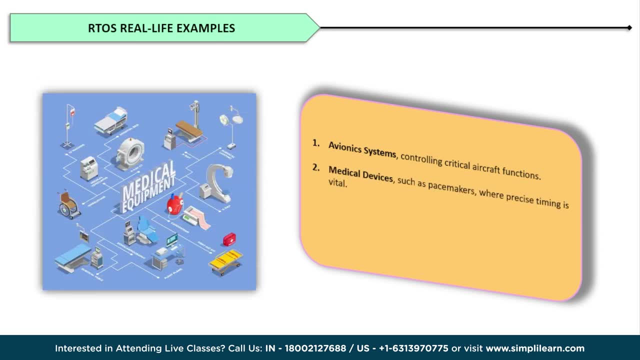 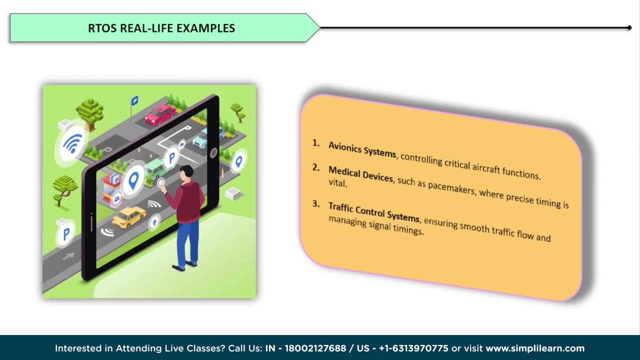 real-time operating system. You'll find them in avionics system controlling critical aircraft functions. They are used in medical devices such as pacemakers, where precise timing is vital. Real-time operating systems are also employed in traffic control systems, ensuring smooth traffic flow and managing signal timings Well before we 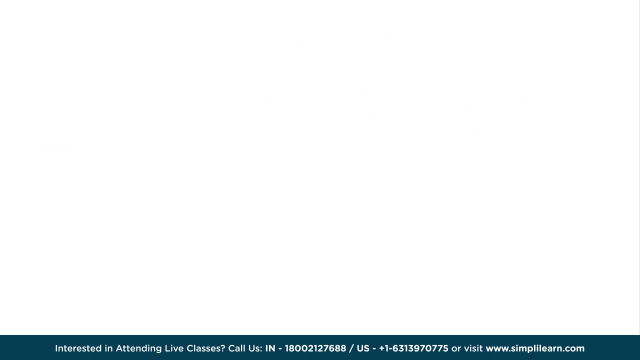 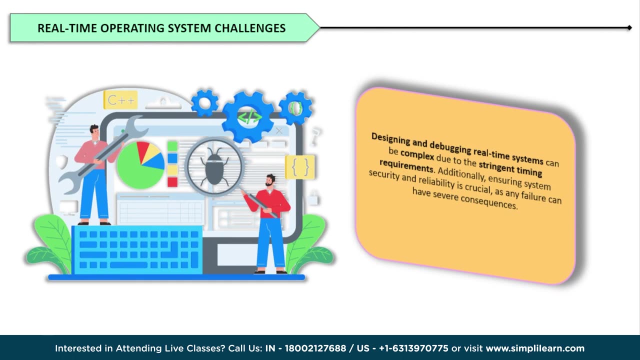 wrap up, let's highlight some challenges faced in real-time operating systems. Deterministic behavior requires careful consideration of hardware and software interaction. Designing and debugging real-time systems can be complex due to the stringent timing requirements. Additionally, ensuring system security and reliability is crucial, as any failure can have severe consequences. 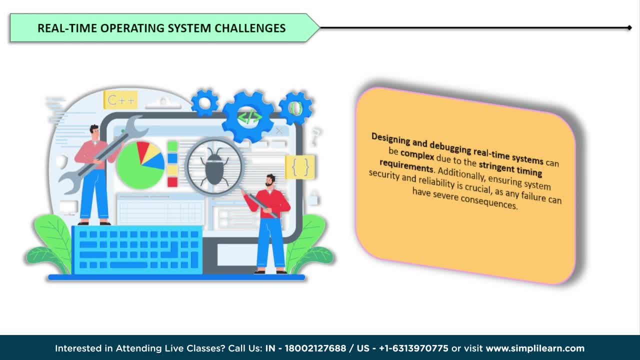 Well. in conclusion, real-time operating systems play a vital role in time-critical applications, ensuring tasks are completed within strict deadlines. They provide deterministic behavior, prioritize critical tasks and respond promptly to events. From automotive to medical and industrial domains, real-time operating systems are powering the technology that keeps 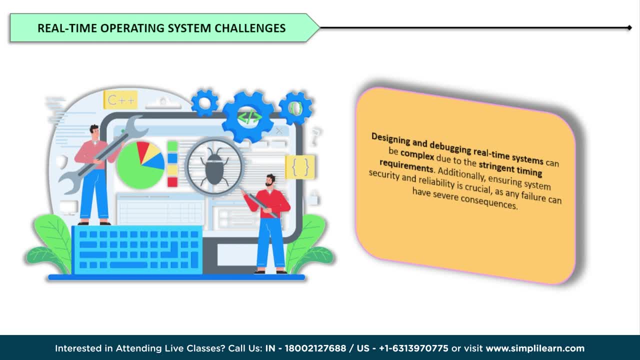 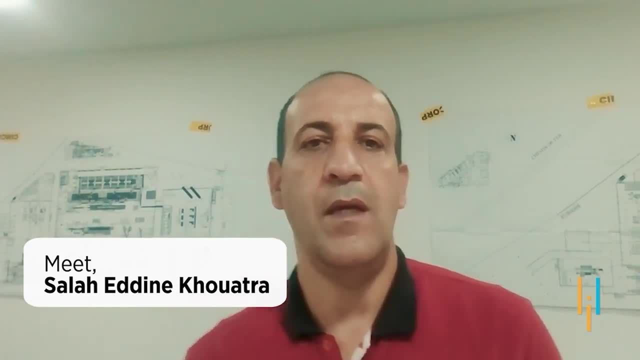 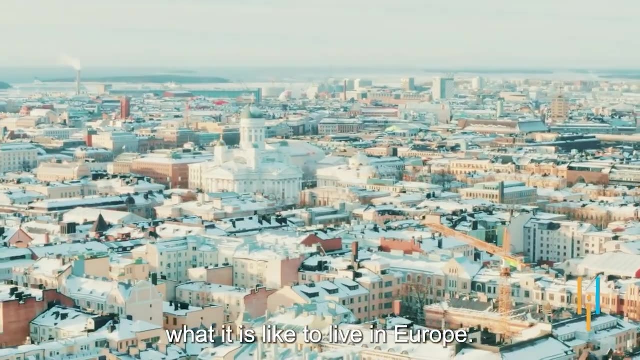 our world running smoothly. Well, here's a success story of one of our learners. to boost your confidence, Do watch this video. Hey, I am Salahuddin Khawatra and I am currently living in Algeria. I wanted to experience what it's like to live in a new country. I also realized that to get a new job, I needed 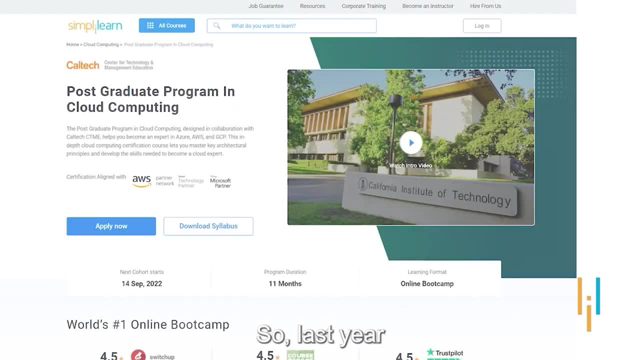 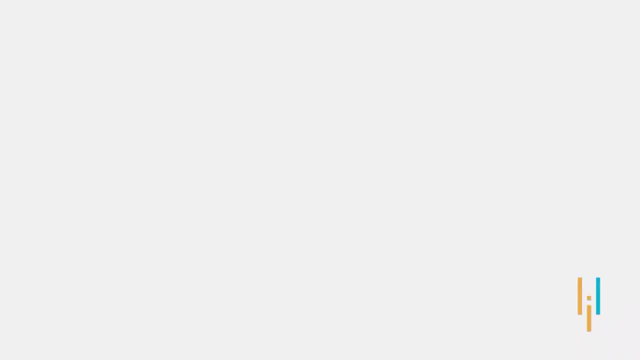 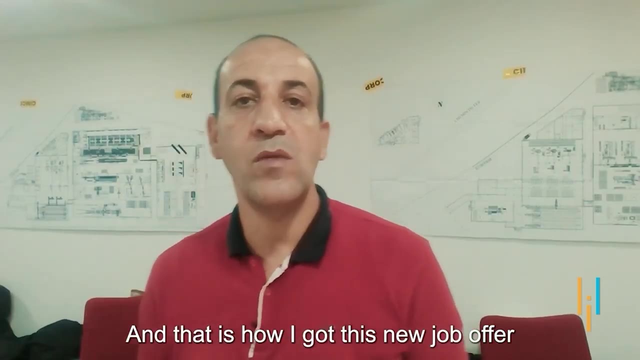 to have a professional certification in cloud computing. So last year I started a postgraduate program in cloud computing in association with Caltech from St William. With this course I had the choice to study while I continued, And that is how I got this new job offer with 60% salary hike In Finland. I will be. 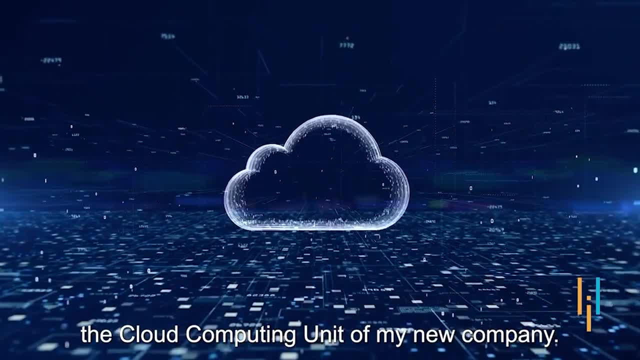 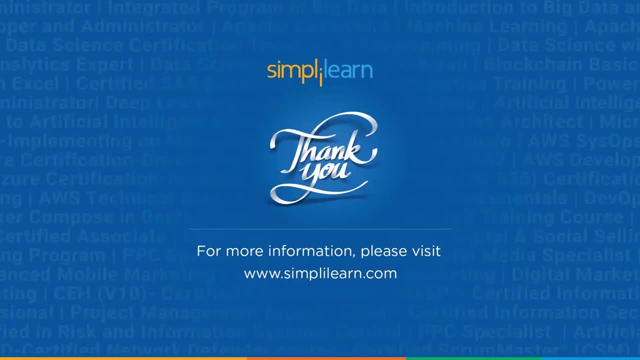 leading the cloud computing unit of my new company. We cannot wait to start our new life in Finland. That's all for today's video. We hope you found this exploration of real-time operating systems informative and engaging. If you have any questions or suggestions for future topics. 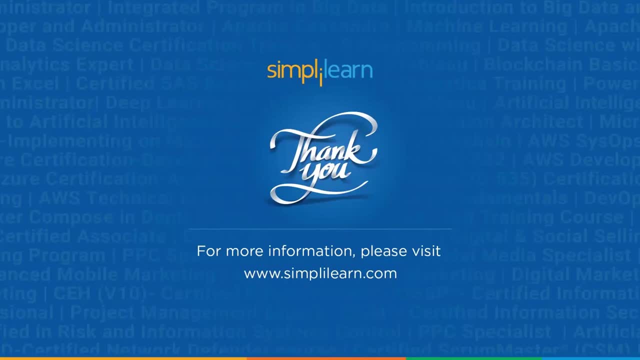 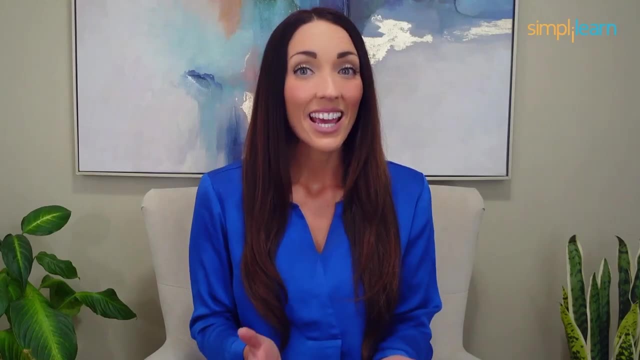 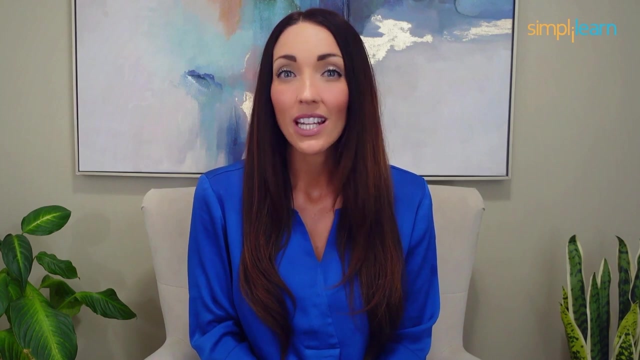 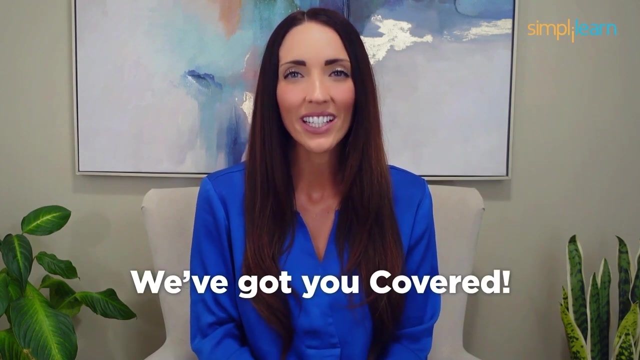 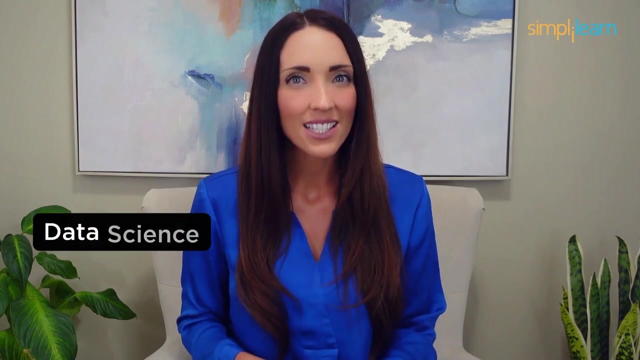 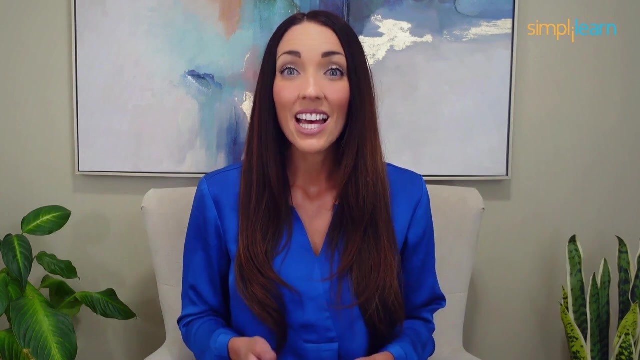 please let us know in the comments section, And don't forget to like and subscribe to our YouTube channel and hit the bell icon for more such interesting videos. Thank you and keep learning Hi there. If you liked this video, subscribe to the Simply Learn YouTube channel.